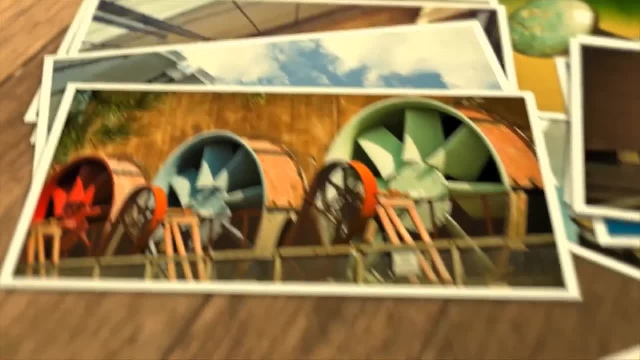 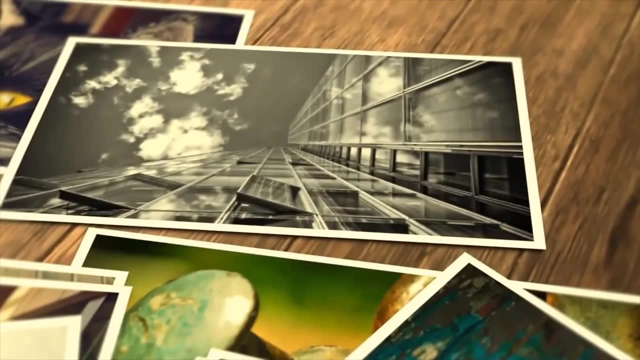 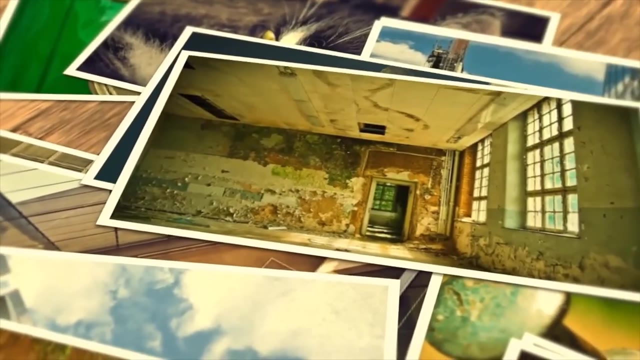 as others will likely have similar ones- To contact us and discuss this or any other environmental issue or to see our services offered. please click the link to our website below And, as always, make your day a good one. 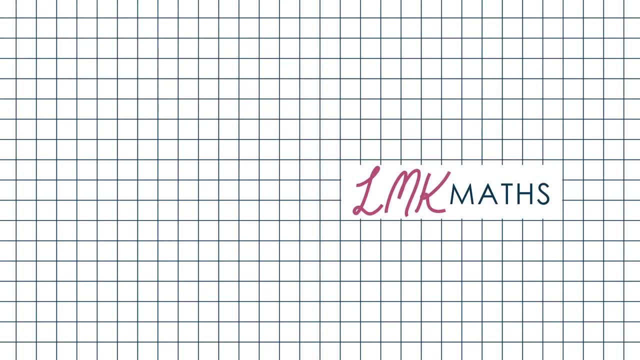 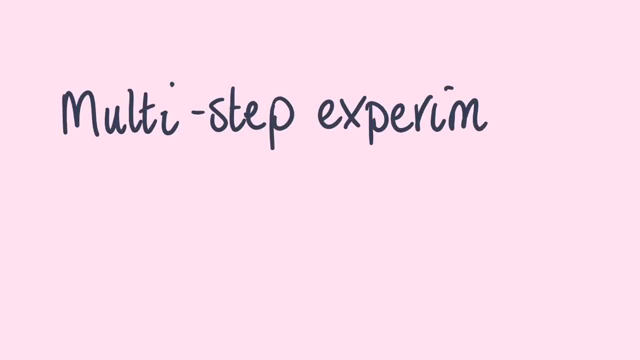 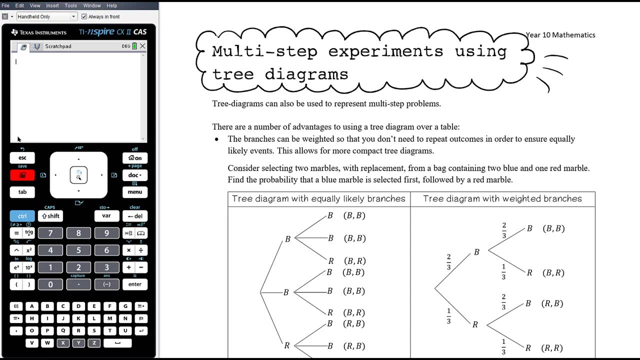 Okay, so in this video we want to continue to look at multi-step experiments, but here we're going to look at using tree diagrams. Generally speaking, I would say tree diagrams work better, but there are certainly examples- and I'll mention one later on- where a table is a. 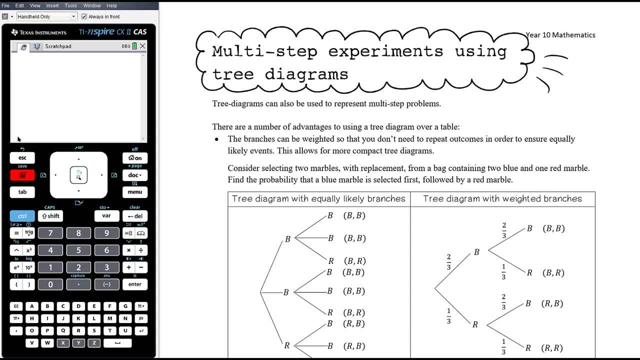 better option. So again, it's about being flexible with your different representations to make good decisions about what's going to be the best way to represent the information in the question, so that then you can find the probabilities required Okay. so there are a number of advantages to using 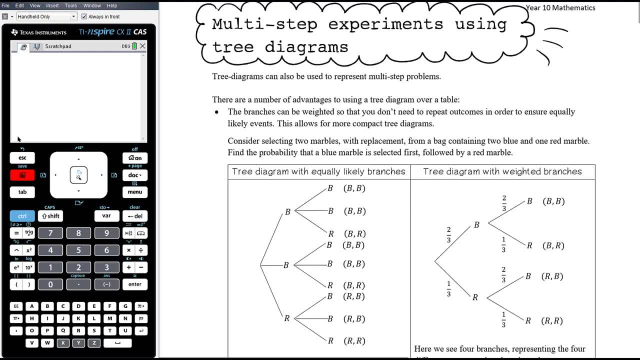 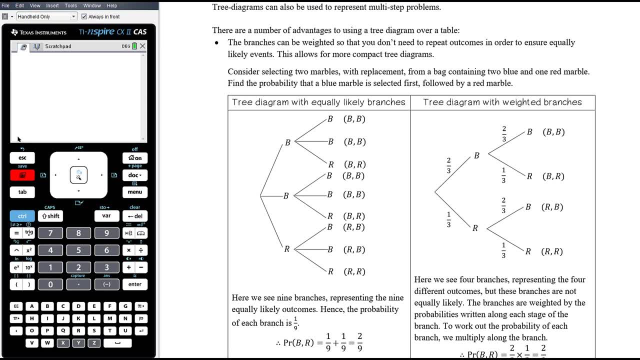 a tree diagram over a table. Okay, so one is that the branches can be weighted so that you don't need to repeat outcomes. So when we did our tables in the previous video, we often had, you know, we had blue, blue, blue red in the columns, because there were three blue marbles and one red and we 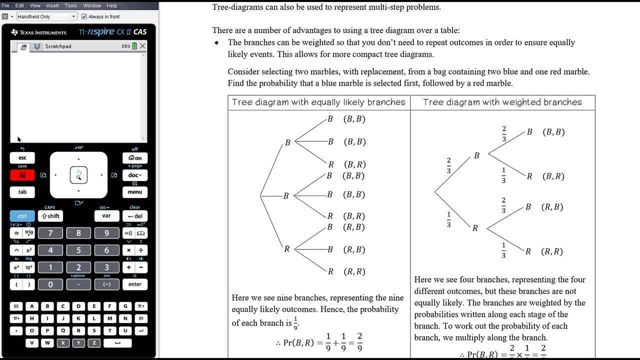 needed to make sure we had equally likely cells in the table. We can set up a tree diagram like that too and have equally likely branches. but we can also condense things by weighting the branches so that we don't need to have such unwieldy tree diagrams. So that's one of the advantages. So if 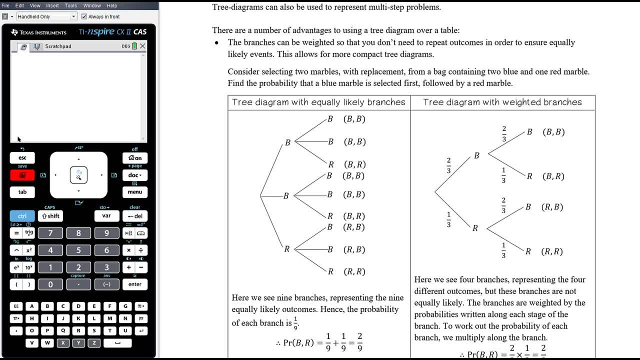 we were to consider a problem where we're selecting two marbles with replacement from a bag containing two blue and one red marble and we want to find the probability that a blue marble is selected first, followed by a red marble, then we could draw this tree diagram over here, which is equivalent.